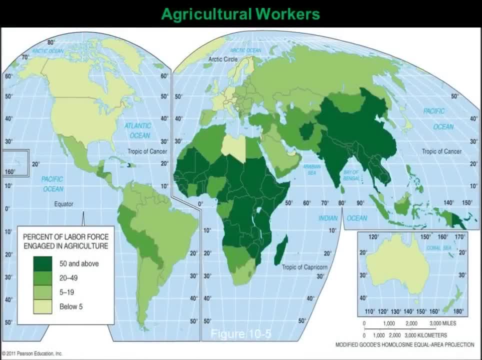 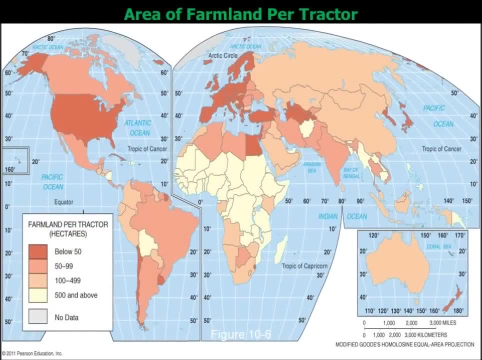 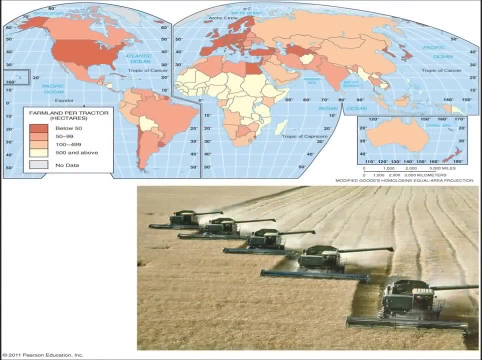 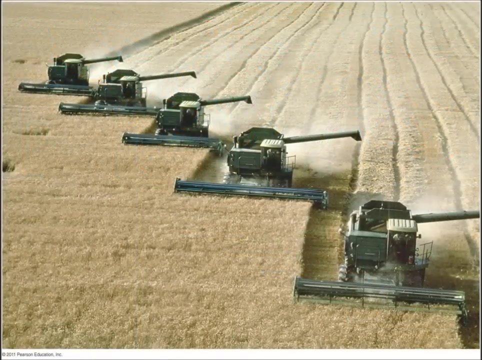 Limited knowledge of alternatives, physical characteristics of the land and climate, And so all those things together are what created different practices. We looked at the role of what has helped MDCs develop commercial farms in the 20th century, And the advantage they have over LDCs would be things like scientific advances, electronics, transportation improvements. 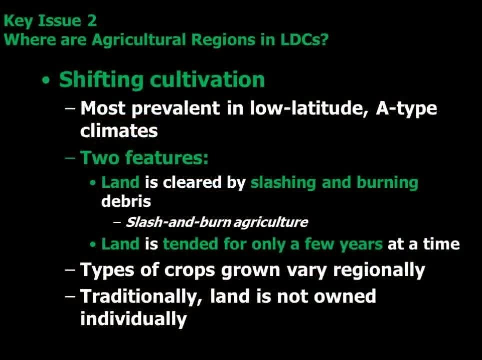 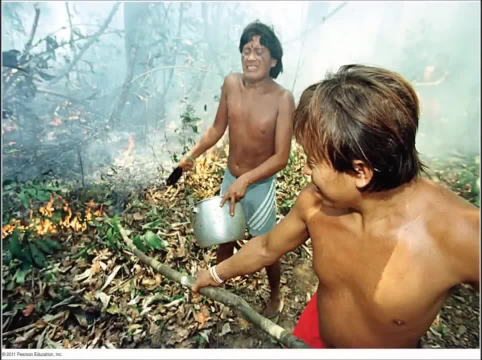 So look at those kind of things, And one of the issues, too that helps In the decline of farmland, especially in MDCs, is the idea of urban sprawl. We looked at different types of farming, For example, subsistence agriculture. 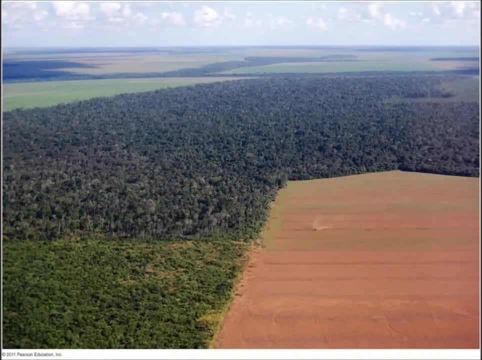 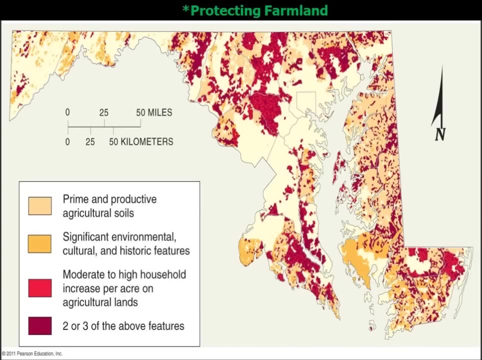 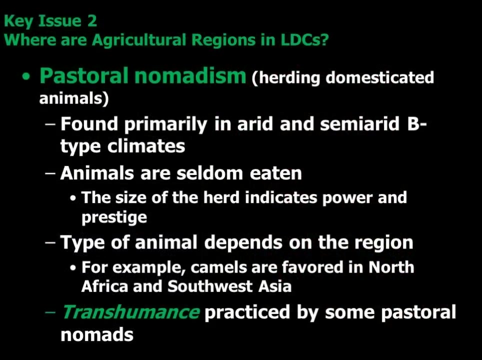 Please know what that is. Please know that we looked at three different types: Shifting cultivation, intensive subsistence farming and pastoral nomadism. Then we looked at the idea of shifting cultivation. Where would you find it? What climate, What region? 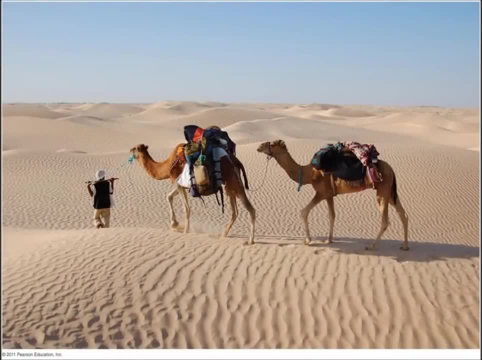 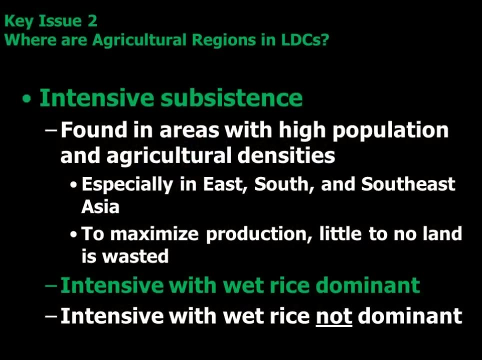 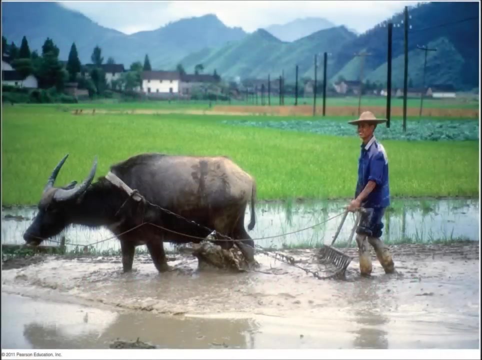 And that would be in a humid or low latitude, where they tend to have high temperatures and abundant rainfall. That's why we can have the floods, the monsoons, for that kind of agriculture. When we look at traditional farmlands and preserving them, one of the key things that is looked at is soil quality. 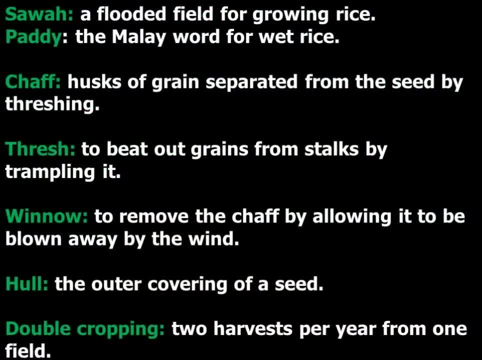 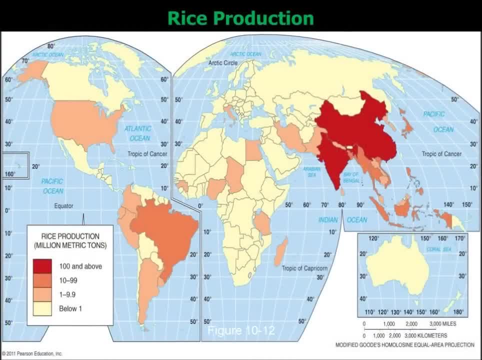 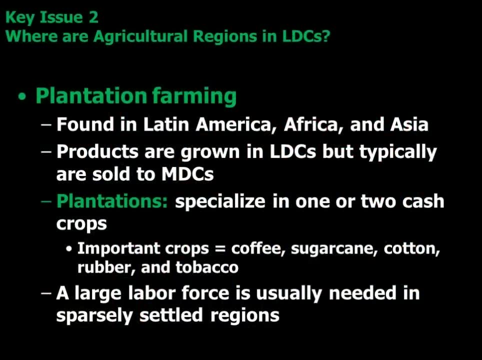 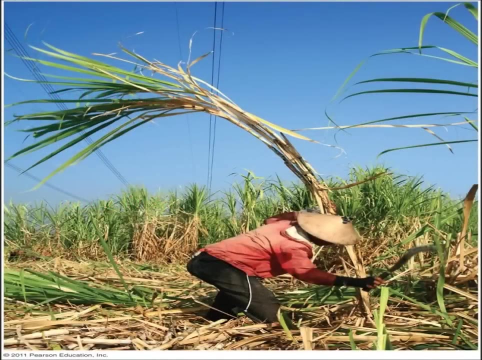 The largest percentage of the people in the world today farm through intensive farming. We tend to see that, and the greatest, largest proportion of farmers of this practice is in Asia. Know the steps of growing rice, from preparing seedlings in the nursery to flooding the land, to plowing the land by oxen and then planting the seedlings in the flooded land. 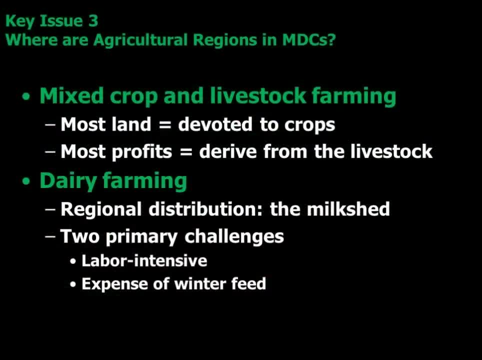 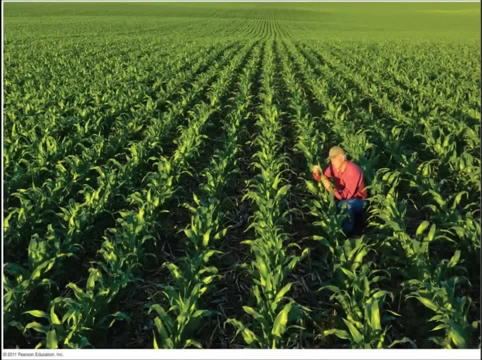 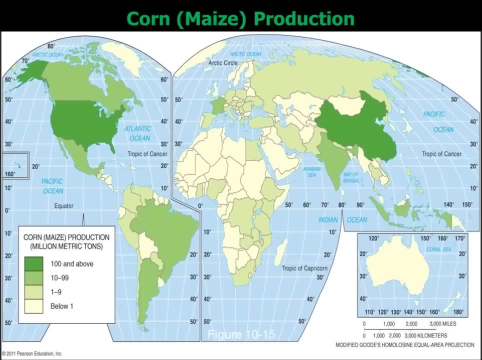 When we looked at China and the different types of crops grown, one of the key reasons, especially for land masses large as China, is their climate. Then we looked at nomadism or pastoral nomadism. One of the key issues for them is their climate and that's why it is done there. 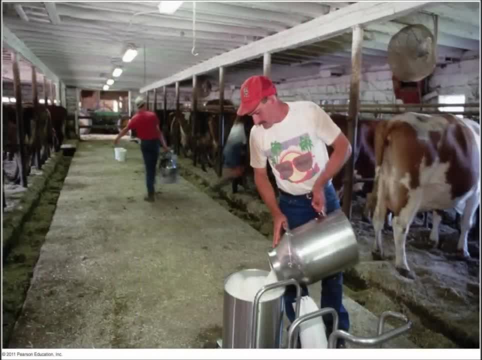 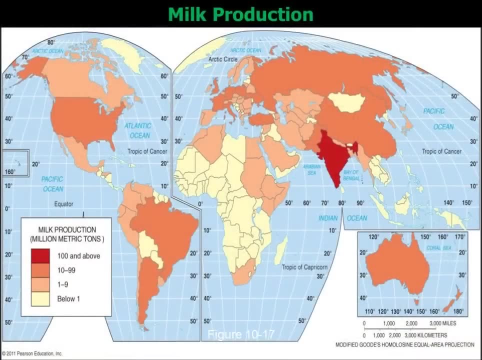 And they live in a dry climate, And this is normally territory or land that they occupy and own. They just move from one region to another. We talked about the term transhumance, and that's the moving of livestock from highlands to lowlands based on weather. 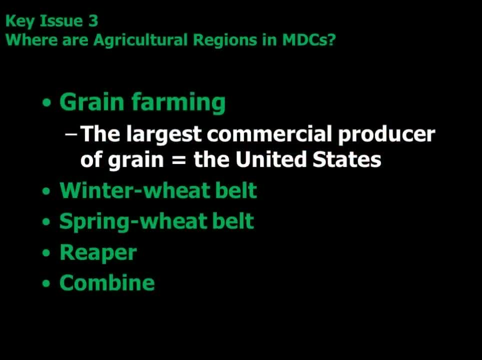 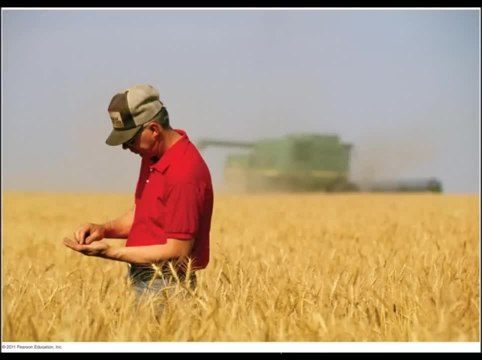 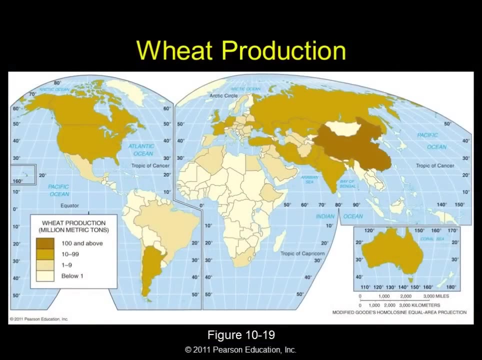 We talked about the idea of double cropping to get more yield from crops, so know what that is. Then we talked about the idea of an MDC's commercial agriculture. One of the key and most common forms is mixed crop and livestock farming. 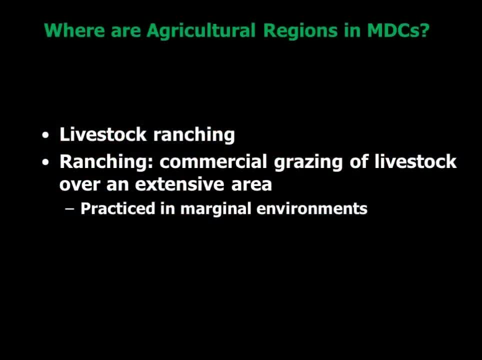 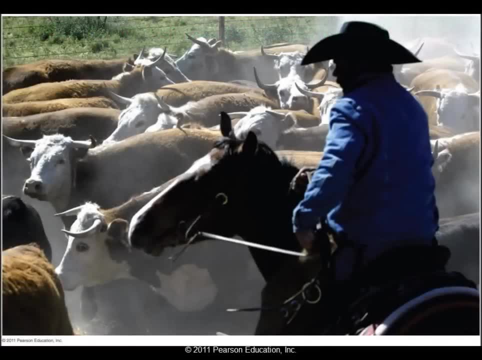 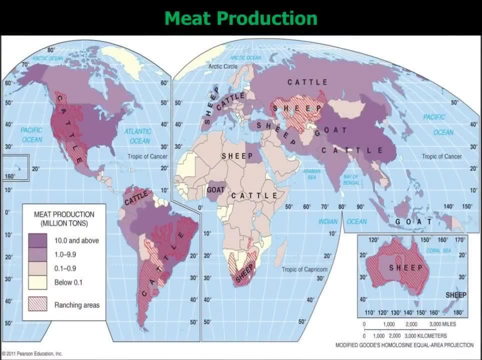 Know what that is, where we're growing both crops and animals and they are helping each other. Know that entire process. We looked at the idea of different seasons of crops, so know the idea, for example, of what is winter wheat and when it is harvested and when it is planted. 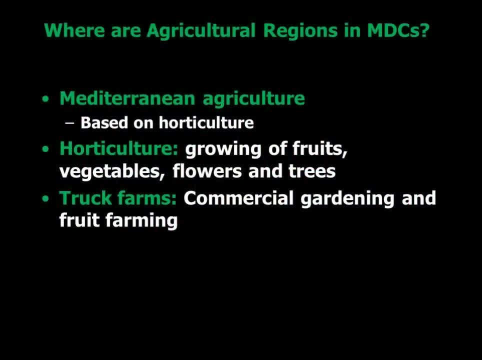 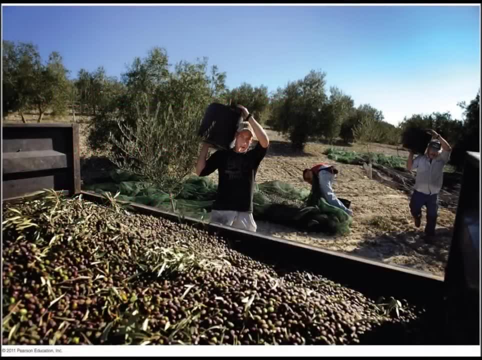 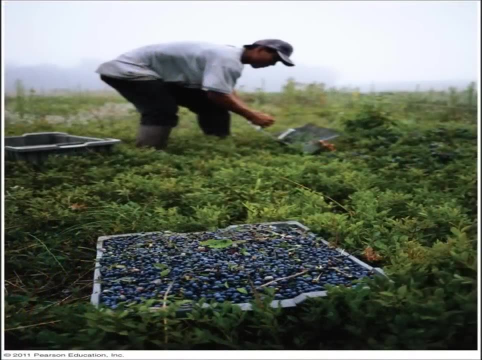 We looked at the idea of agribusiness, which is what the United States is very a way of looking at our farming, and that's when it's integrated in the entire food production industry. That's one reason why ranching has declined in this country. 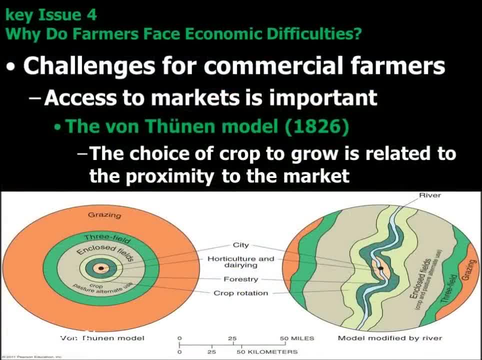 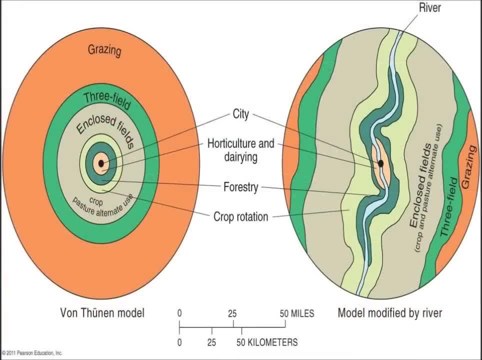 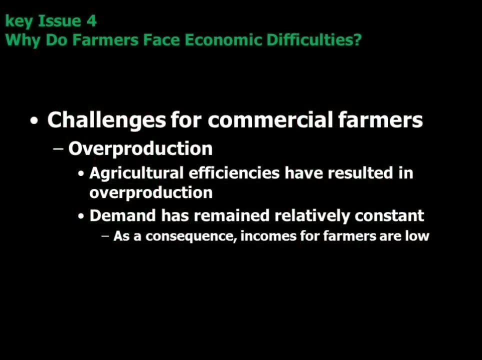 Due to crops yield more profits than the cattle and easier to deal with in many cases, And if you compare ranching, it's very much like pastoral nomadism. We looked at the idea of Mediterranean agriculture so know what type of products are grown and what is least likely. 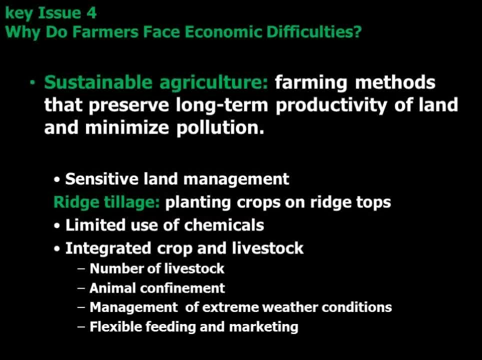 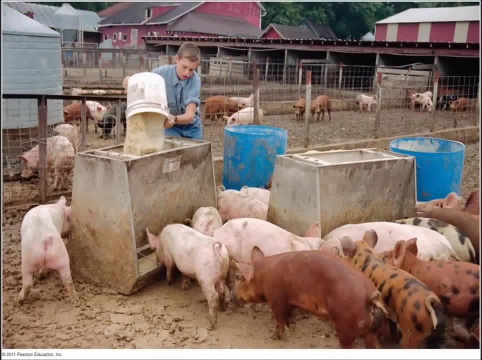 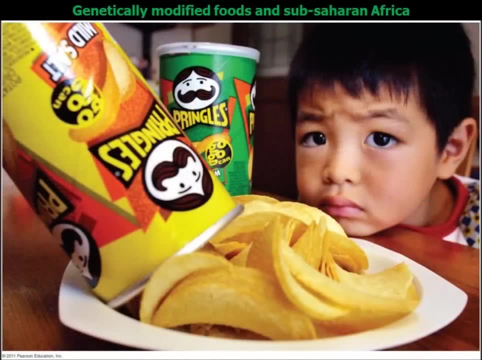 Much more: fruits, cereals, olives, grapes, those kind of things. Look at the idea of why we use cropping, The idea of rotation And the idea of sustainable agriculture, where we use integration of crops and livestock. We don't use very many chemicals. 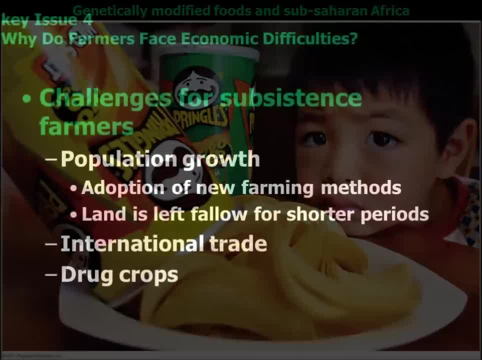 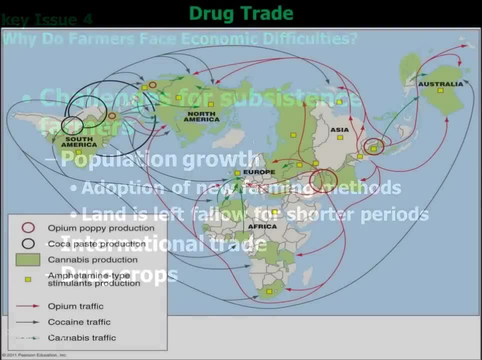 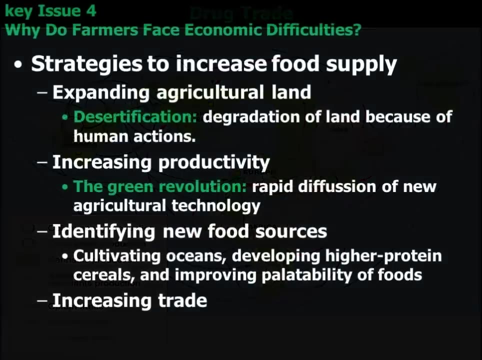 We're sensitive to land management, Those kind of things. Then we looked at Von Theuen's model for choosing commercial farm products And the whole key there is market location And how far from market can I have my products so that they won't perish before I can get them to market? 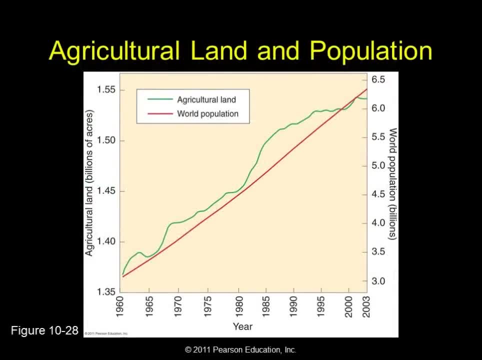 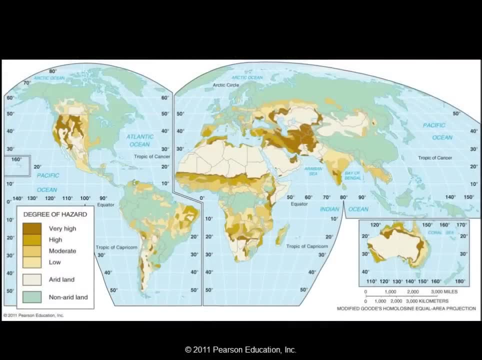 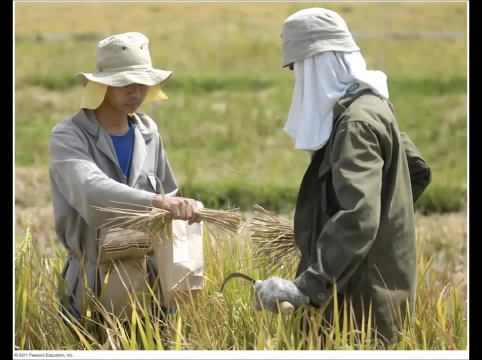 And how easy it is to transport them to market. Then, finally, the last idea is looking at some of the videos we looked at And, as the chapter also talks about differences from MDC's and LDC's, what crops they choose to grow,